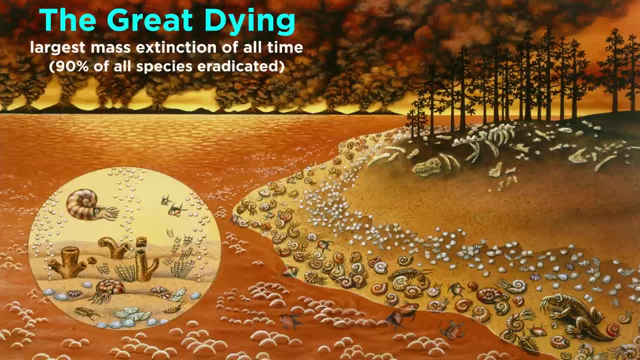 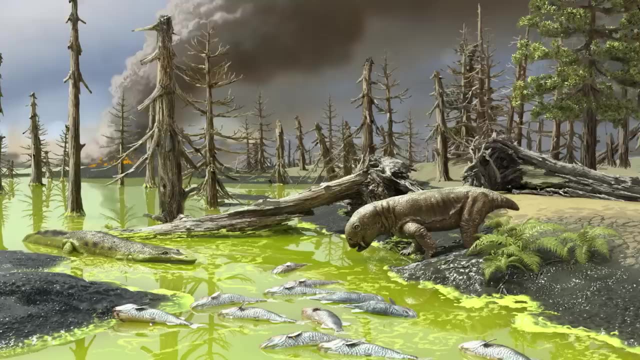 and acidification, causing the extinction of over 90% of the ocean. This was the largest mass extinction event of all time and is known as the Great Dying. Only time will tell if an event of such magnitude will be repeated. After the end Permian mass extinction, life immediately began to recover and evolution 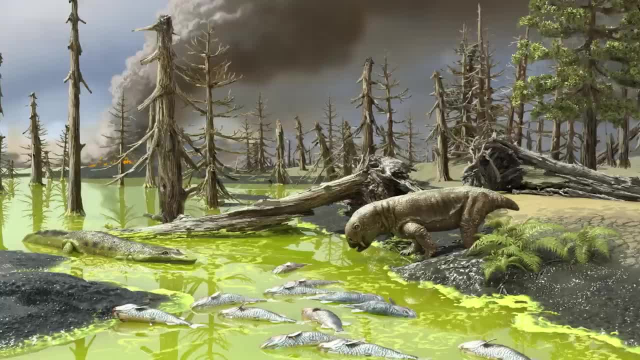 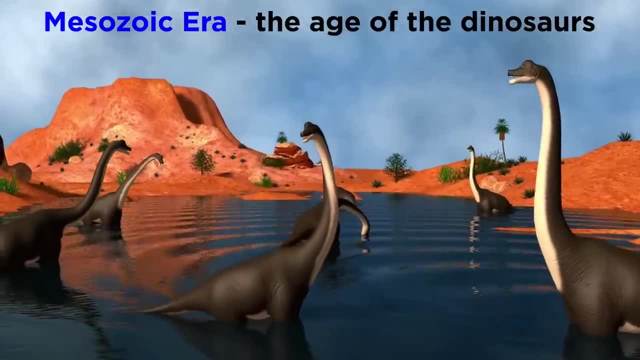 kicked into high gear, taking advantage of increased living space and reduction of predators. Thus began the Mesozoic Era, which is known as the Age of the Dinosaurs, Since they had evolved and subsequently took over Earth. during this time, In addition to the evolution, 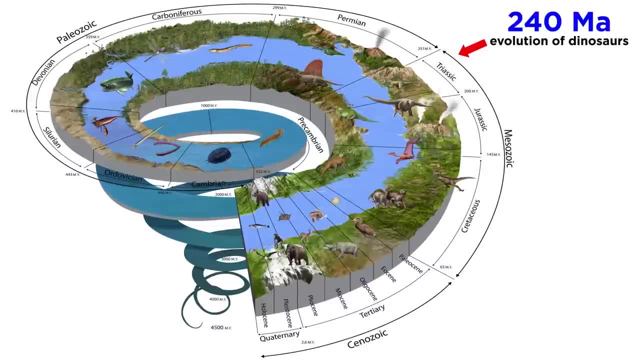 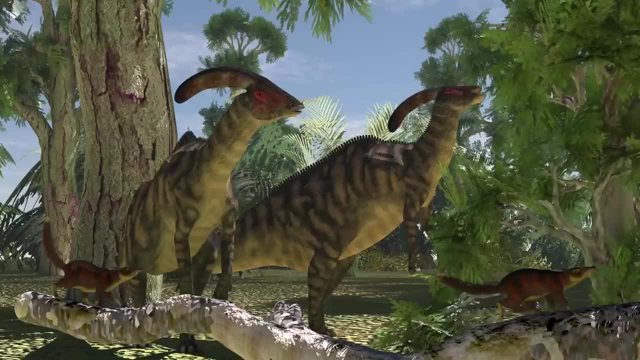 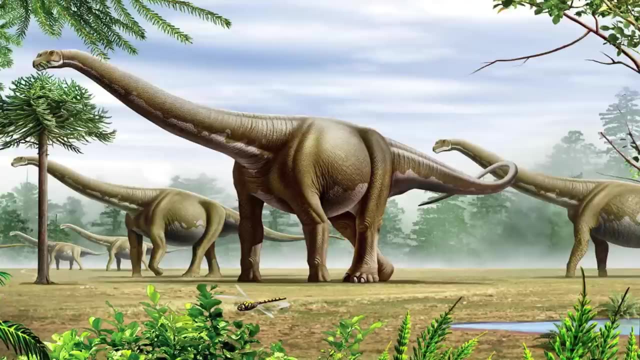 of dinosaurs, which occurred around 240 million years ago. mammals also evolved during the Mesozoic, but around 30 million years later. This evolutionary head start helped the dinosaurs dominate the mammals throughout their existence. For a long time, dinosaurs were imagined to. 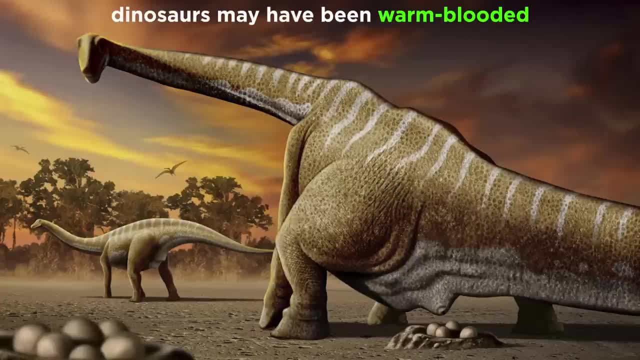 be enormous lumbering creatures, but recent discoveries suggest that they may have been warm-blooded. They were believed to have lived for a long time and they could have been meaning. they could raise their body temperature in cold weather, allowing them to be more active. 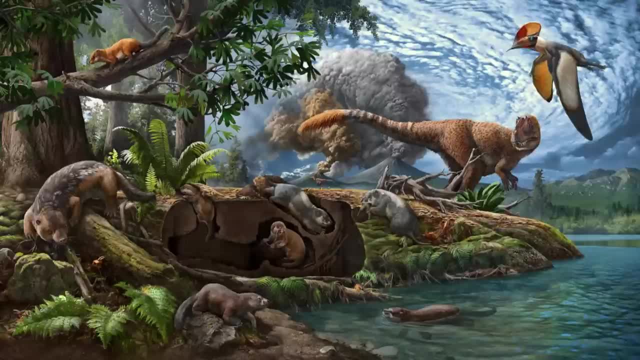 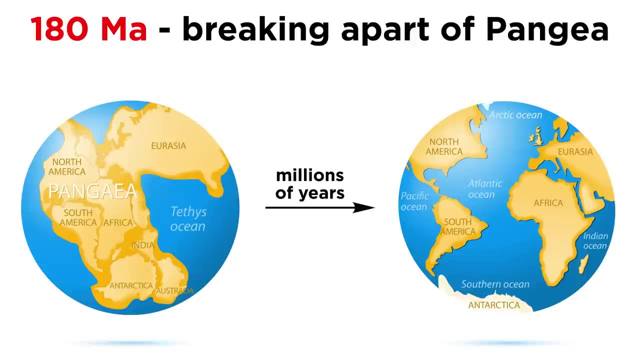 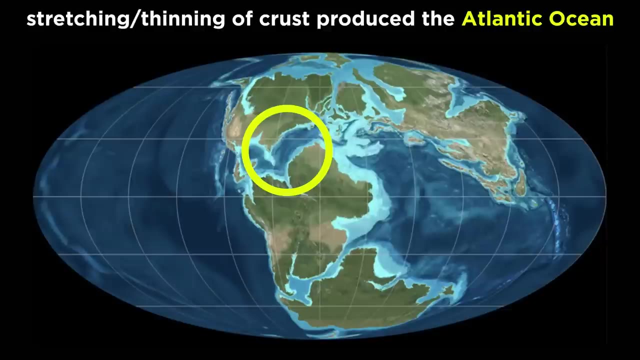 than any other animal. at that time at least, until the evolution of mammals. The most impactful tectonic event of the Mesozoic era was the breaking apart of Pangea, which began around 180 million years ago. The axis along which Pangea broke apart would go: 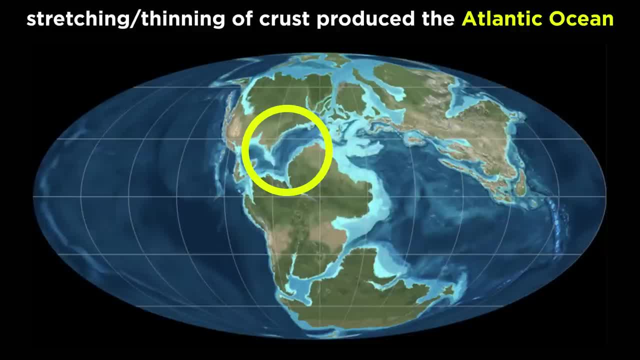 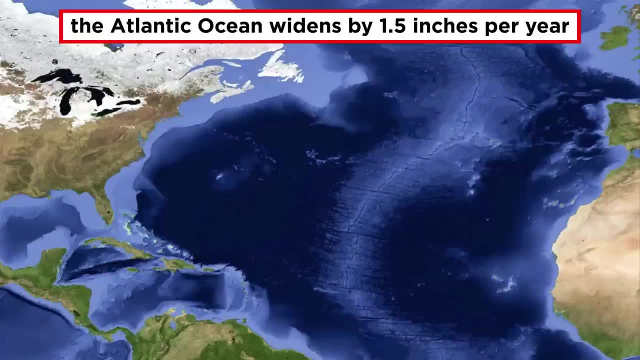 on to become the Atlantic Ocean as the crust was stretched and thinned down to below sea level. due to the divergent motions of the mantle below, The Atlantic Ocean continues to widen to this day as new oceanic crust is created along its axis, where hot upwelling mantle rock partially melts. 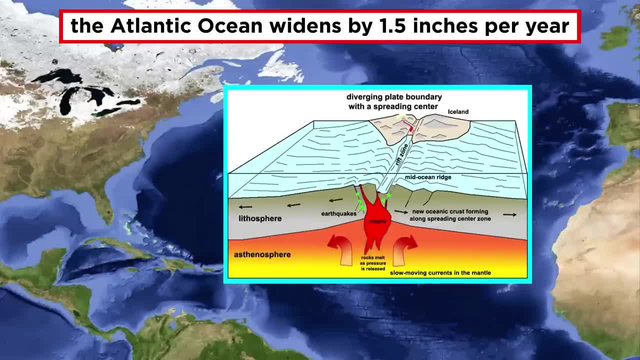 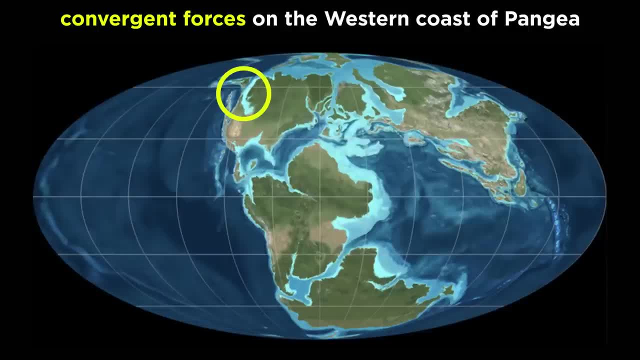 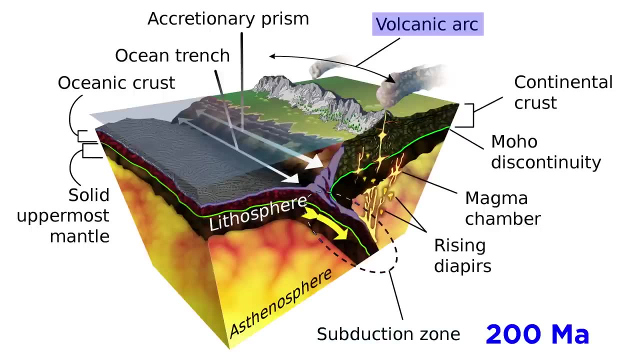 and solidifies near the surface of the ocean floor. Along the western coast of North America, which was also the western coast of Pangea, convergent forces dominated and a new subduction zone was created around 200 million years ago. This would begin a theme of continuing cycles of mountain building. 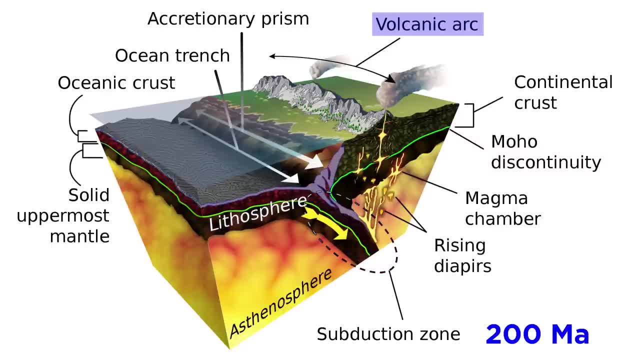 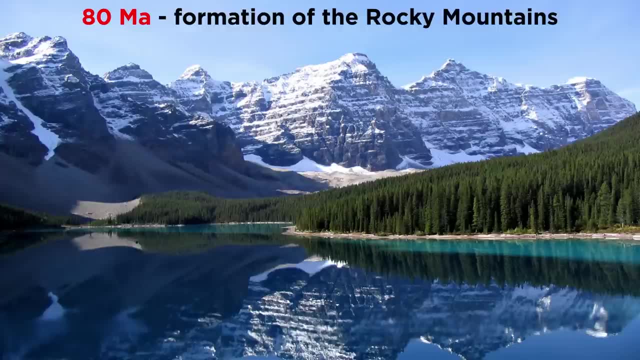 and volcanism that have also lasted until present day. This convergent plate boundary was responsible for uplifting the Rocky Mountains, which began forming around 80 million years ago. As we wrap up the Mesozoic era, some experts say that the Mesozoic era was a time when the Mesozoic era was a time when the 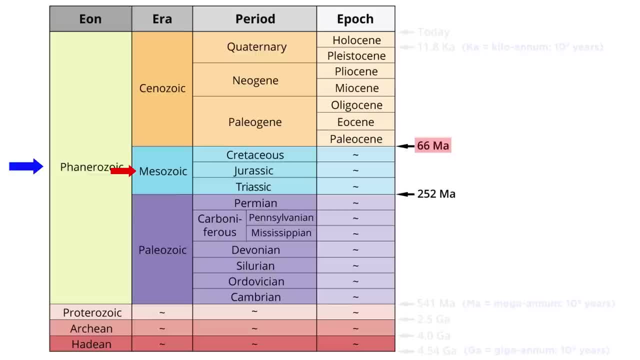 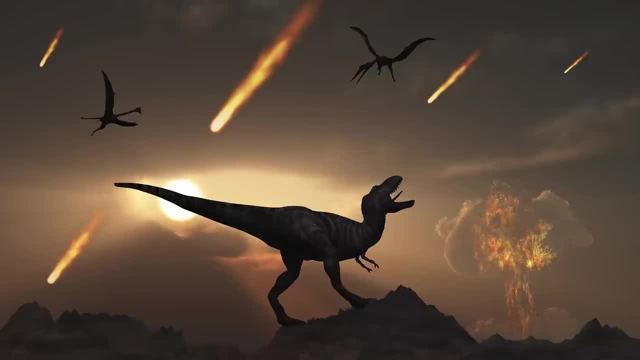 extraterrestrial trouble is on the way that will change the Earth's biosphere forever. The Mesozoic era ended with another mass extinction event, but this one was not of an earthly origin: An asteroid with a mass equivalent to about 50 million Titanics. 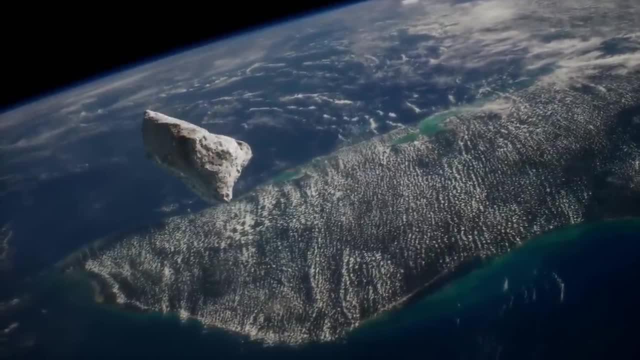 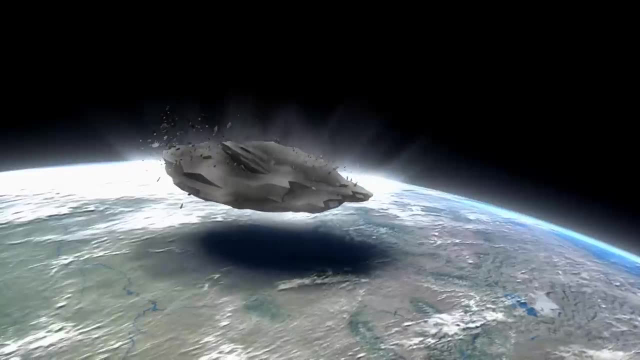 slammed into Earth near the present-day Yucatan Peninsula. The impact itself was equivalent to a 100 million megaton bomb. The thermal pulse from this impact instantly came to an end. The impact itself was equivalent to a 100 million megaton bomb. The thermal pulse from this impact instantly came to an end. 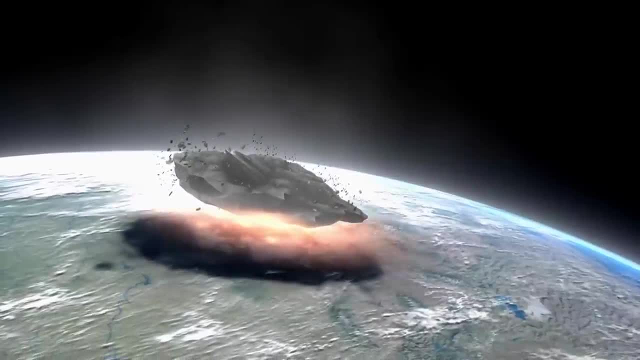 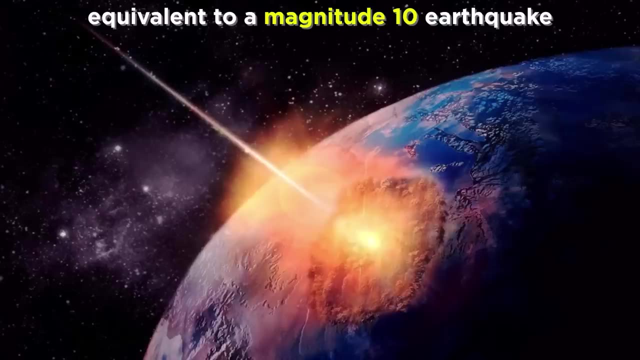 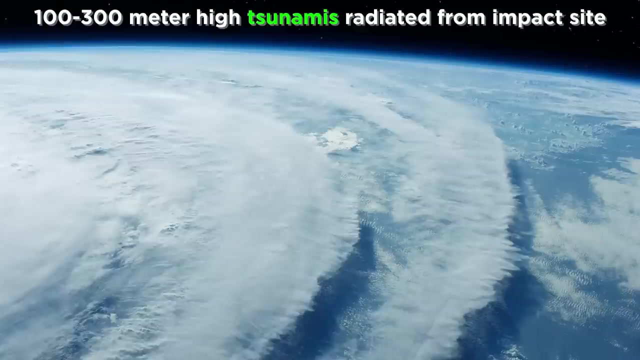 The earthquake killed anything nearby and the shockwave created hurricane-force winds extending out about 1,500 kilometers from the blast site. It was a seismic event equivalent to a magnitude 10 earthquake, Because the asteroid impacted the ocean tsunamis 100 to 300 meters high. 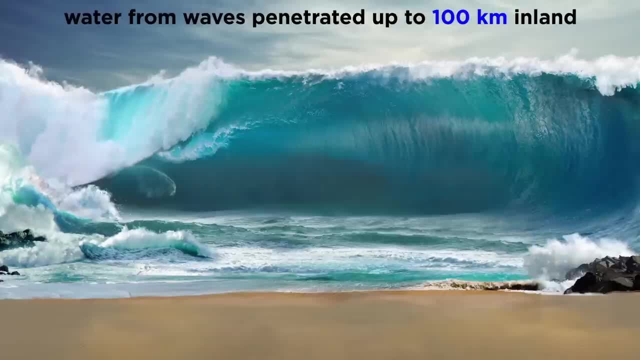 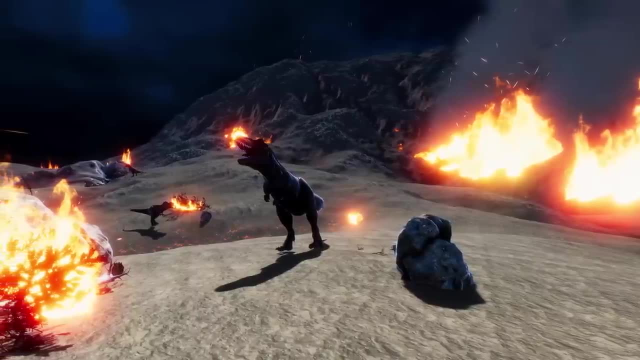 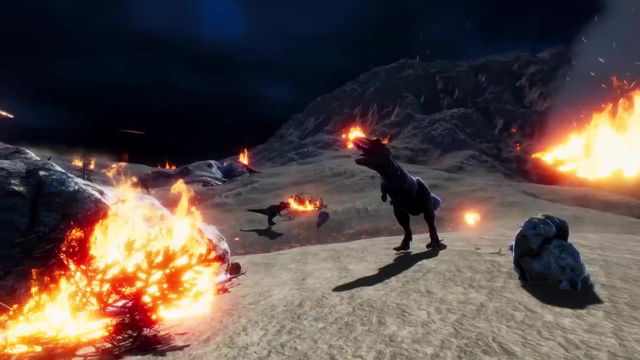 radiated across the Atlantic, crashing along coastlines and penetrating up to 100 kilometers inland. Molten fragments of Earth were ejected into the atmosphere upon impact that, upon returning to the surface, would heat Earth's surface to hundreds of degrees Fahrenheit: devastating. 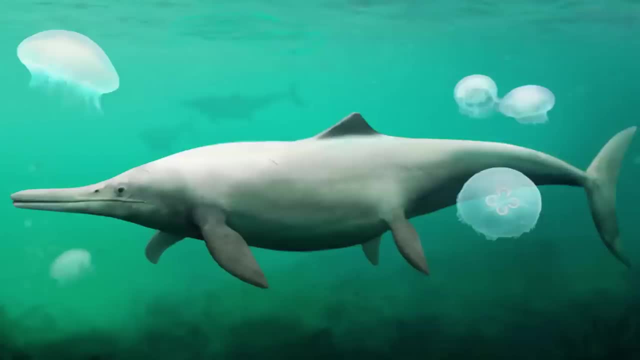 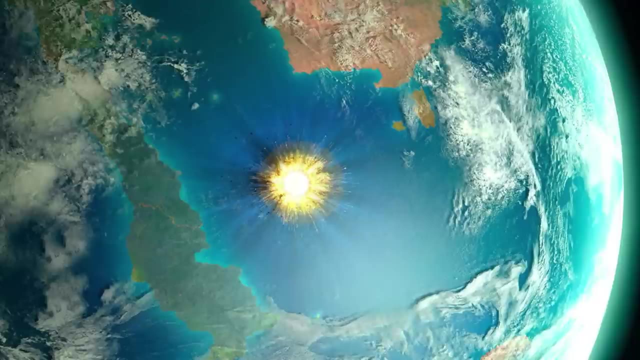 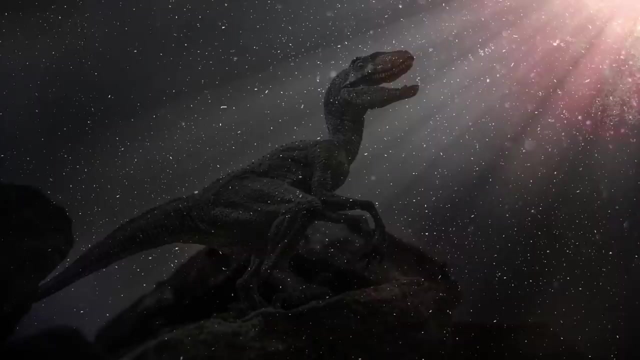 terrestrial plants and animals, but sparing most marine life due to the high heat capacity of water. The combination of these events obliterated life proximal to the impact site, but the real worldwide devastation would come from long-term consequences. Dust particles were blown into the atmosphere and the earth's surface was destroyed. The dust particles were blown into the atmosphere and the earth's surface was destroyed. 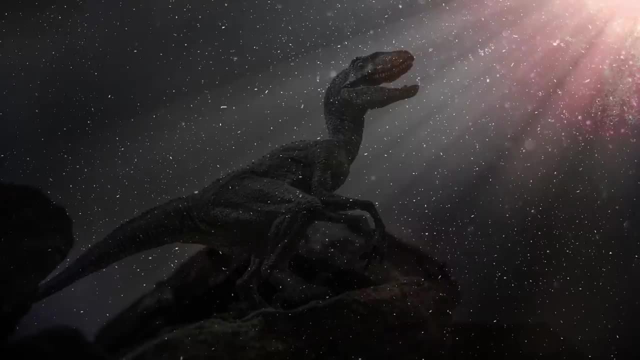 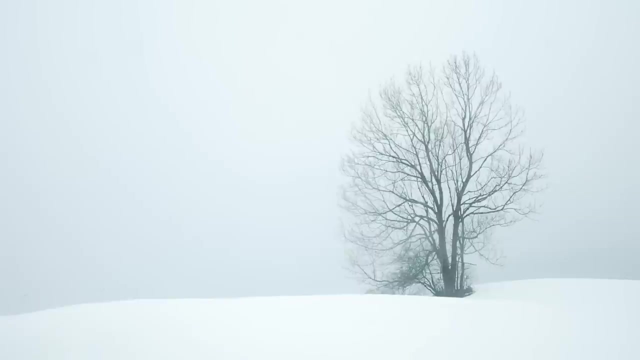 Where they remained for months. This blocked off sunlight, causing both perpetual darkness and a global winter. This several-month period of darkness would have likely killed off anything that relied on photosynthesis for energy, which would then travel down the food chain as herbivores. 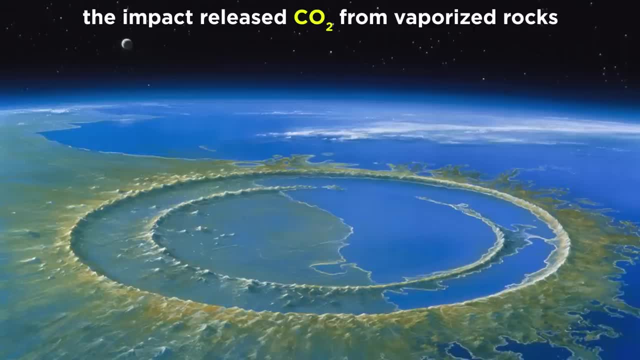 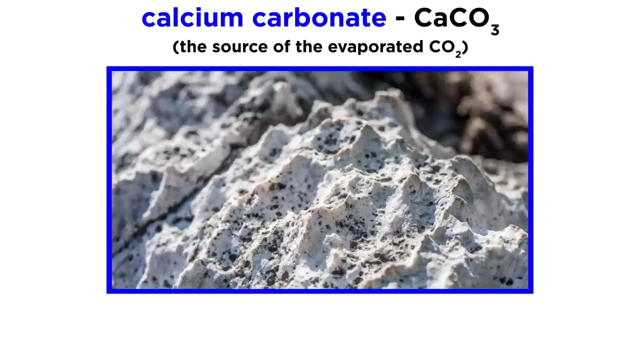 ran out of food. However, the longest-term effect of the impact was the global warming associated with CO2 released from vaporized evaporite rocks Which precipitated from the evaporation of ocean water. These rocks were primarily composed of calcium carbonate, the source for the CO2, and calcium sulfate, which vaporized and reacted.